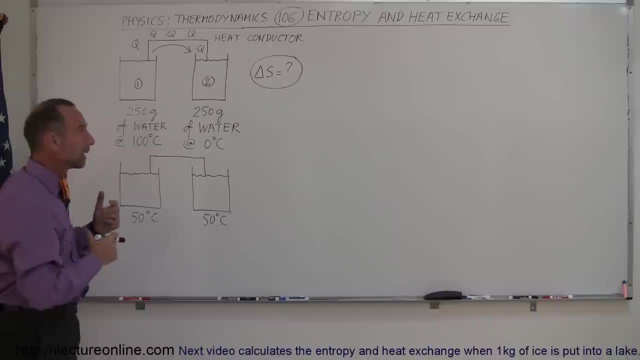 In this next example on entropy, we'll be able to get a better understanding by showing how this works over here. So here we actually have a heat exchange, We have a hot cup of water- 250 grams- It's about a quarter of a quart. 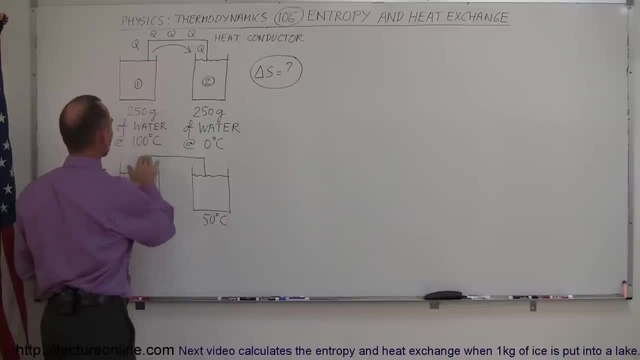 And we have a cold cup of water- same amount, 250 grams. The hot cup is 100 degrees centigrade, The cold cup is at 0 degrees centigrade And there is a heat conductor that connects to two cups so that heat can travel from the hot cup to the cold cup in those little cues that represent heat traveling from one to the other. 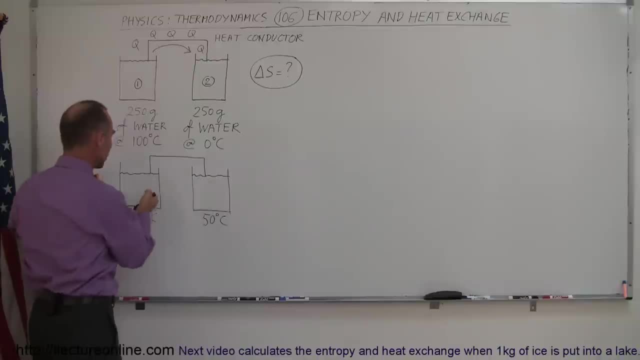 And eventually they both will be at the same temperature. This one will cool down, This one will heat up And since they have the same amount of water in them, they will actually both end up at 50 degrees centigrade, providing no heat is lost to the environment. So make it simplistic. 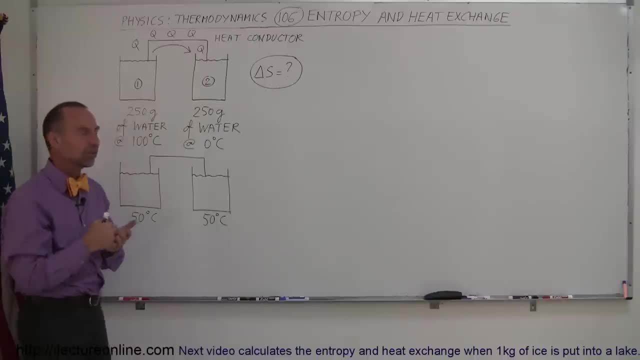 And in this heat exchange we're going to have a change in the entropy And, of course, as we expect, we expect that to be a positive We've changed. Entropy always goes up when there's an exchange of heat, So how do we calculate the amount of the entropy change? 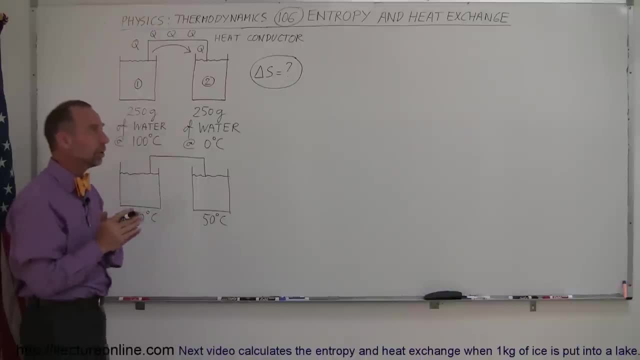 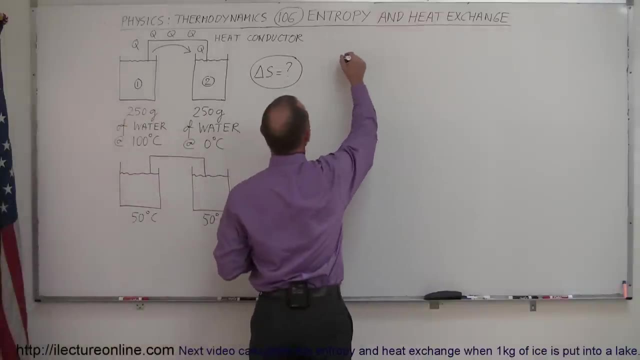 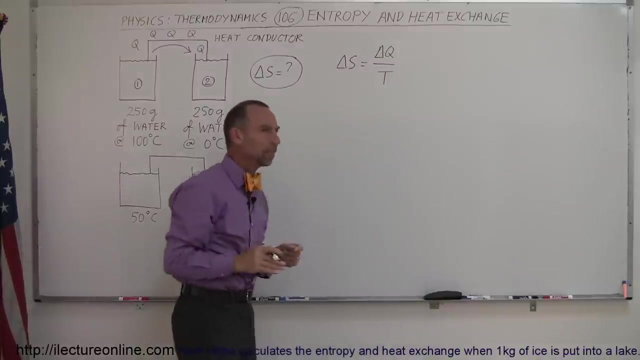 Well, since the temperature is changing, we probably want to use the integral of that in the form that I use- the integral, But I think we can find a simplistic way of doing it. So if we say that the change in the entropy is equal to the amount of heat being exchanged divided by the temperature at which this happens, 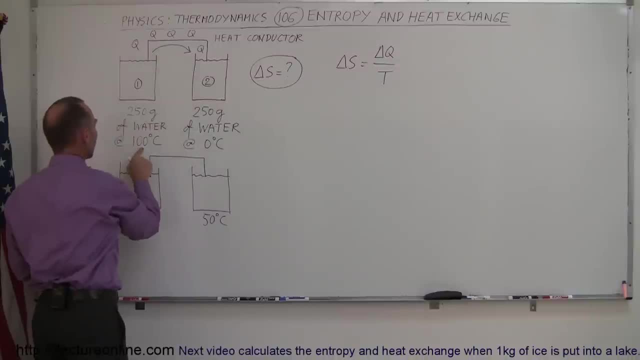 And notice. let's take cup number one first. That starts at 100 degrees Centigrade and it ends at 50 degrees centigrade, So it's a relatively small change in the temperature And if we take the average temperature during that exchange, we come up with a pretty close value, a pretty accurate value, using that equation rather than the integral. 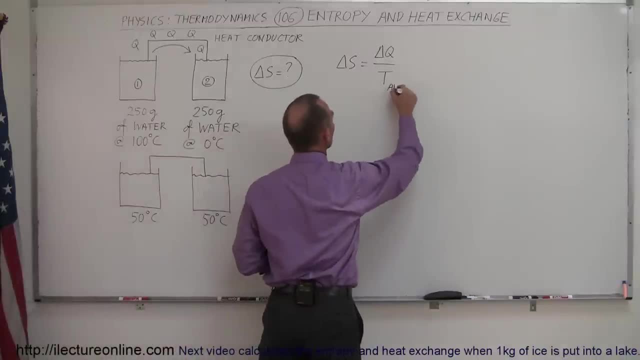 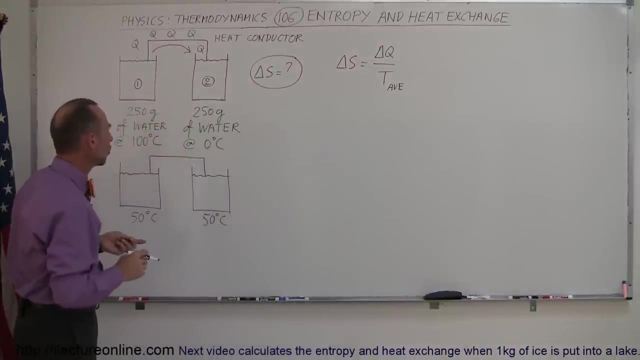 So let's go ahead and do that. So we're going to use the average temperature. Now, that is a good approximation. that usually gives you a very good answer. All right, Now how much heat was exchanged? Well, the water changed from 100 degrees centigrade to 50 degrees centigrade. 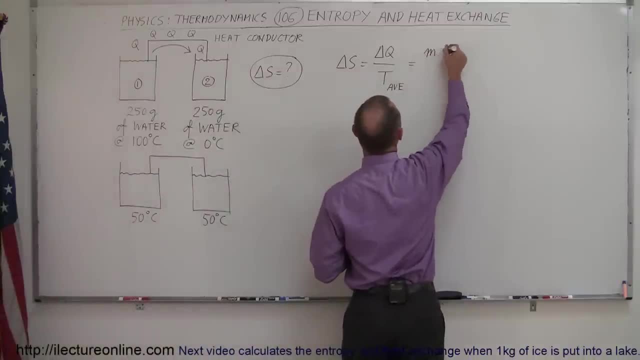 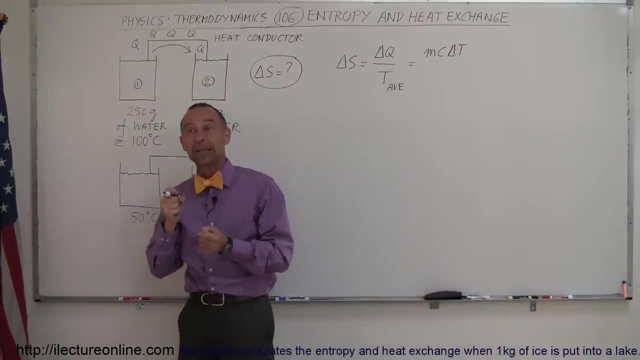 So the delta Q is going to be? It's going to be equal to mc delta t. Now, is that going to be positive or negative? Well, since we're taking heat away from the cup, that has to be a negative quantity. 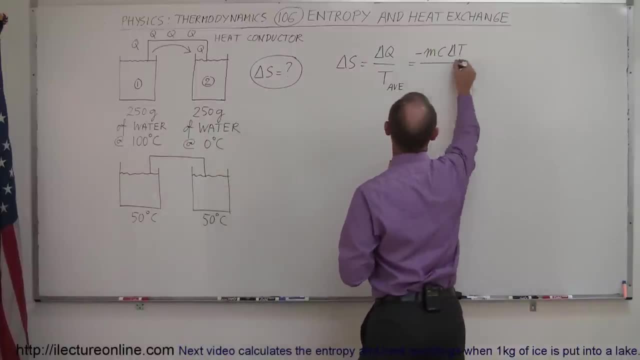 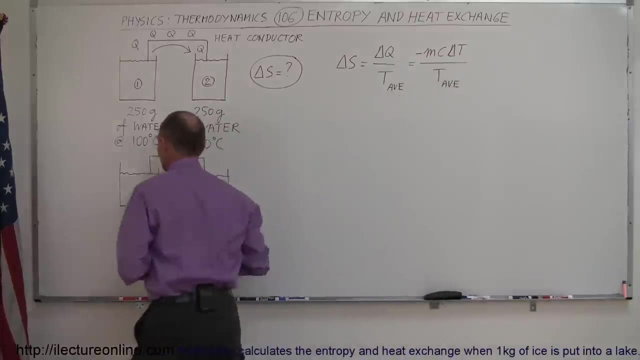 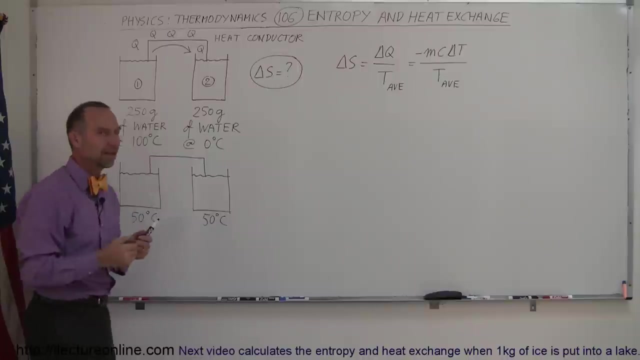 So it needs to be a minus mc delta, t divided by the t average at which this occurs- t average. Now, another way in which you can do this is not worry about the negative sign and simply say that the final temperature is smaller, The initial temperature is greater. 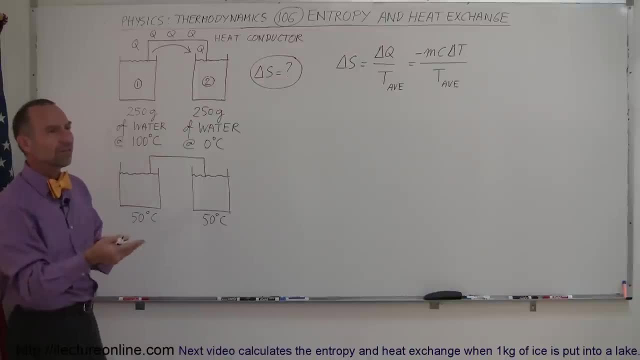 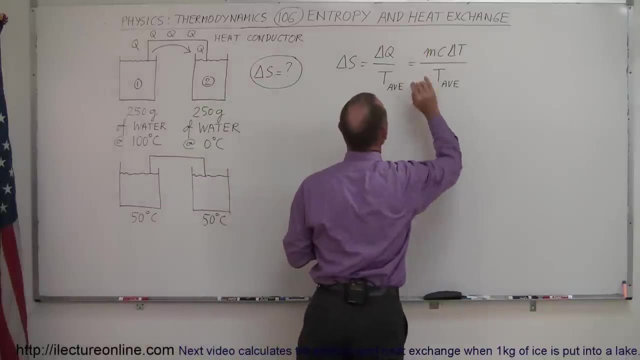 And if you then of course subtract Delta t can be written as t final minus t initial. That means you'll get the, automatically the negative sign. So we can think about that and say, OK, we don't need to worry about that if we just strictly stay with the proper delta t. 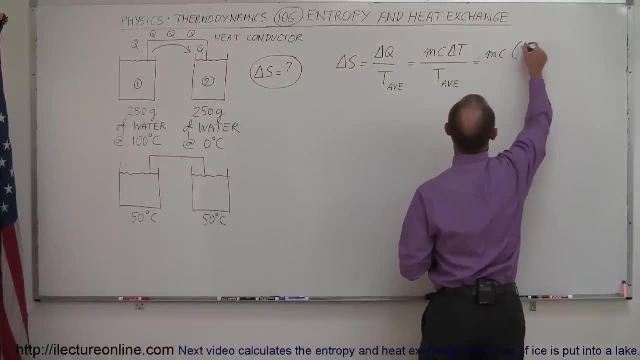 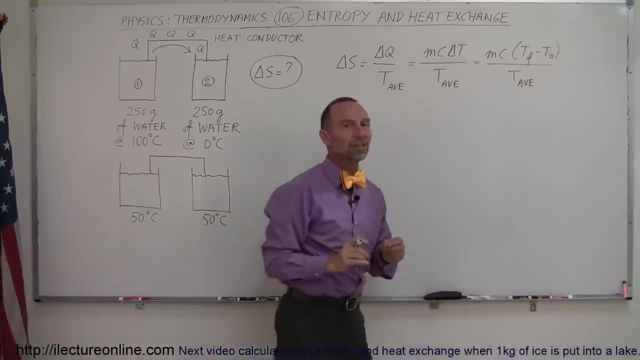 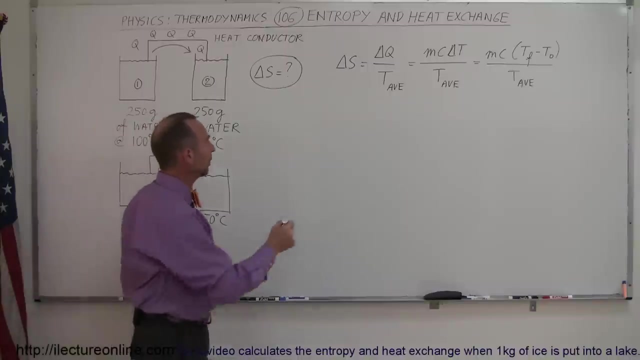 In other words, we're going to write this as mc times t final minus t initial, divided by t average, And then that will automatically give us the negative of the heat exchange. All right, Let's plug in the numbers that we have. So this is: 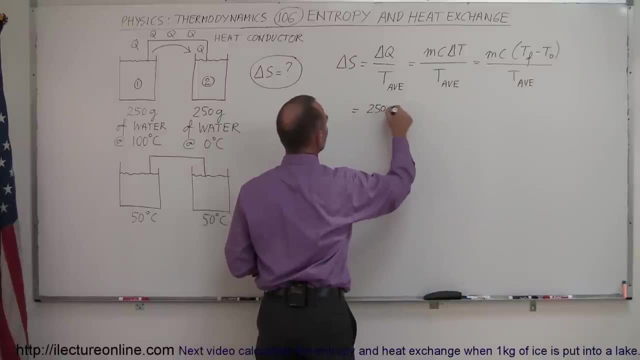 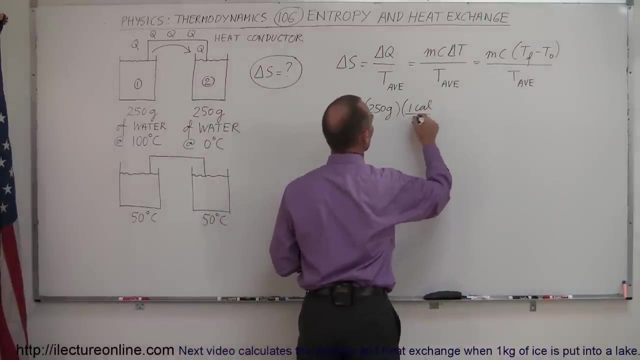 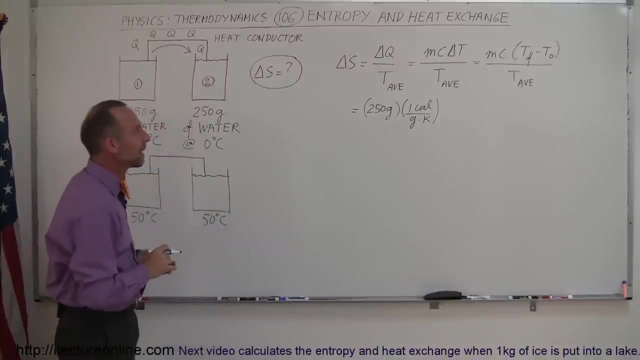 This is equal to the mass, would be 250 grams times c. Now for water, c is one calorie per gram per Kelvin centigrade degree. centigrade centigrade degrees or Kelvin, Same thing. And times t final minus t initial. 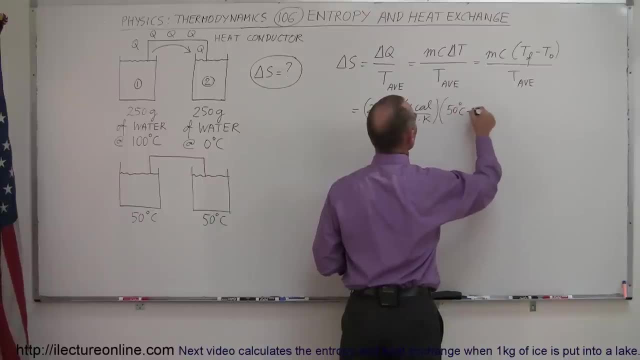 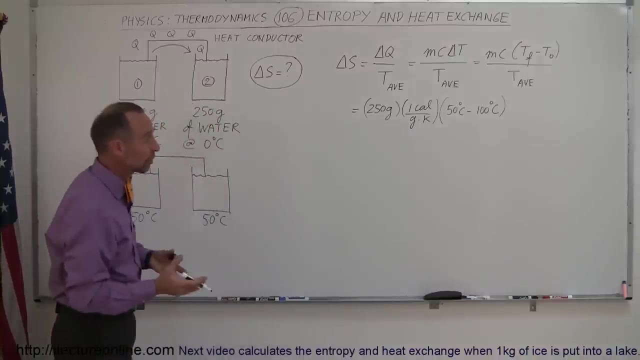 So it would be final would be 50 degrees centigrade minus 100 degrees centigrade. Now we don't have to convert that. It would be Kelvin per se, because Kelvin degrees and centigrade degrees are about the same size. 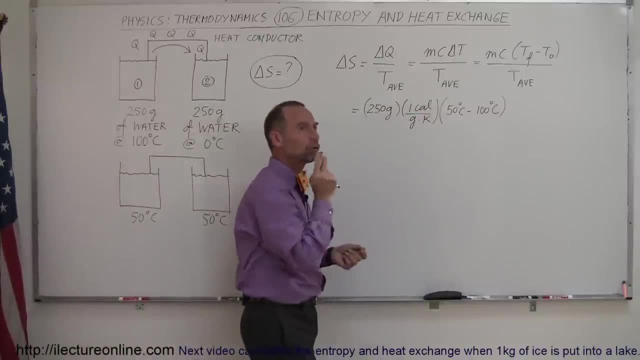 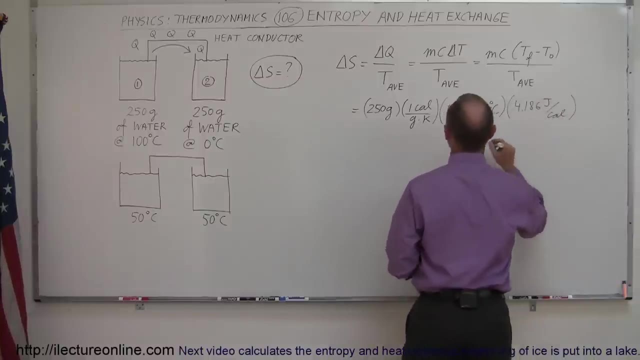 Now we do have calories in there and we want to convert that to joules. So we need a conversion factor of four point one, eight, six joules per calorie. So now we can see that calories disappear, grams disappear, So we don't have to worry about that. 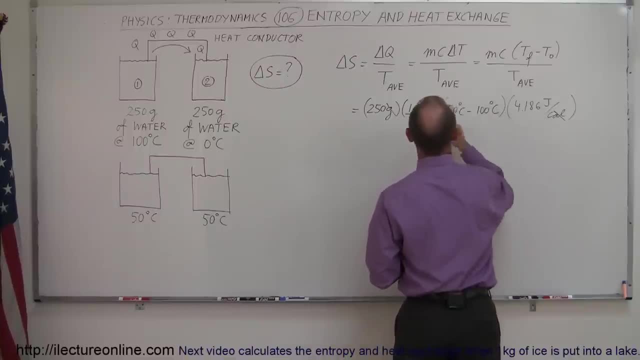 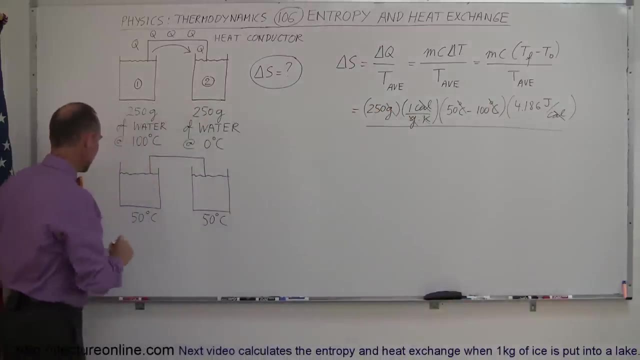 And then we have centigrade degrees and Kelvin degrees, So that cancels as well. We still have to divide that by the average temperature. Now the average temperature would be. Let's see here: in this case, t average would be equal to seventy five degrees centigrade. 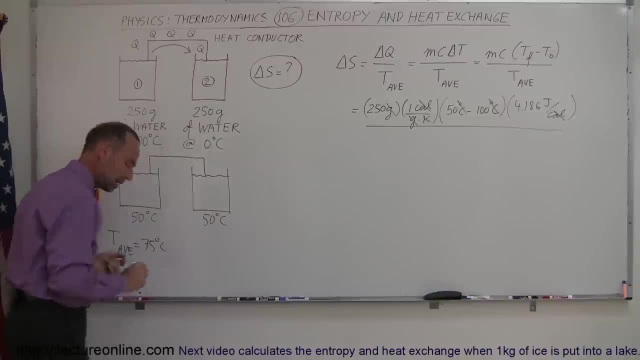 which converted to Kelvin. we have to add that to two hundred seventy three. So let's make sure we get that right. Two seventy three plus seventy five, That would be three hundred and forty eight Kelvin. All right, So we divide that by three hundred and forty eight Kelvin. 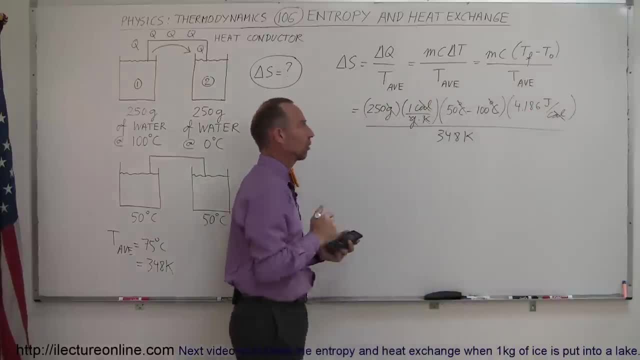 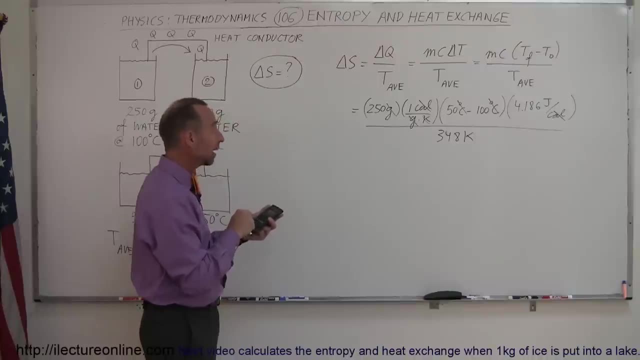 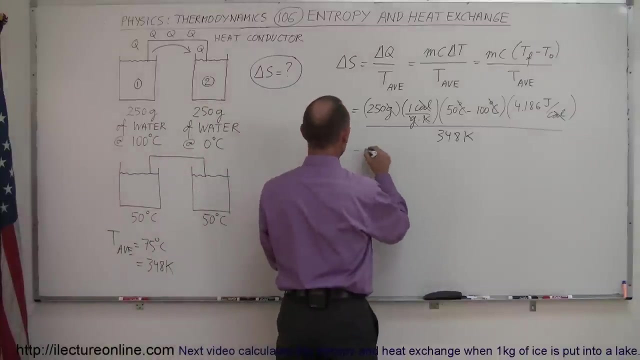 And now you can see the units are going to be joules per Kelvin And that's correct. So 250 times A negative, 50. Times four point one, eight six, and divided by three, forty eight equals, and that would be a minus one hundred and fifty point four joules per Kelvin. 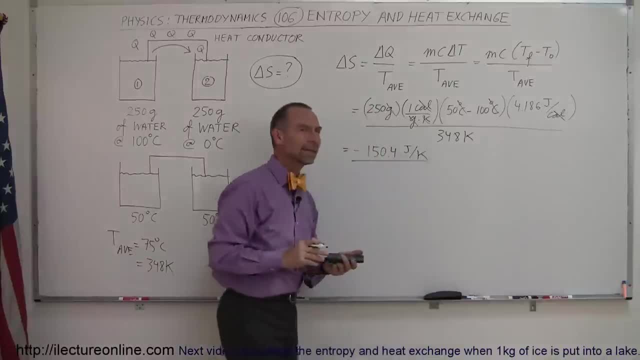 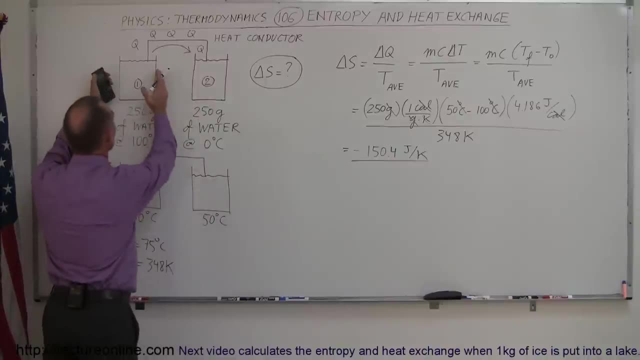 Now notice it's a minus, And you say: well, wait a minute. didn't you just tell me that the change in entropy is always positive? How do we get a minus out of that? Well, that's only for this part of the process. 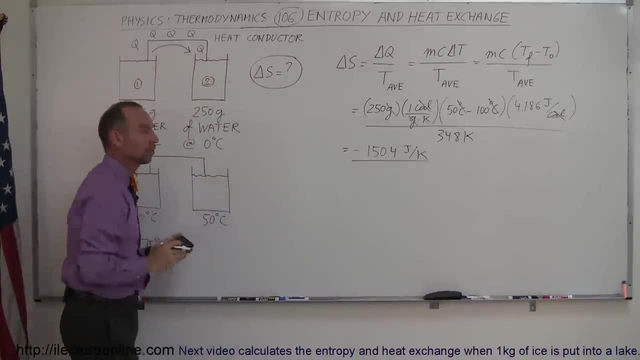 We still have to find the change in the three For this part of the process. So now this was for one. Now we have to do the same for Delta S, for part two. That's the cup that receives the heat, And since it's receiving heat that Delta S will be positive. 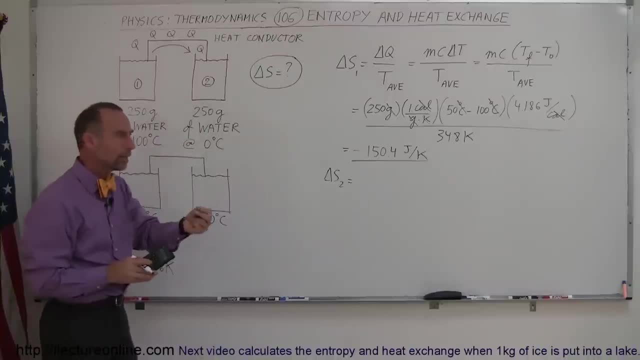 And since it happens at a lower average temperature, that will be a greater quantity. And you see that a greater positive quantity will negate a smaller negative quantity. You'll see in just a moment. All right, So again we have 250 grams of water in the cold cup. one calorie per gram per. 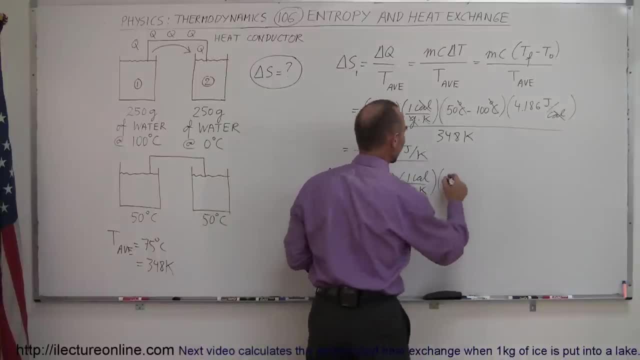 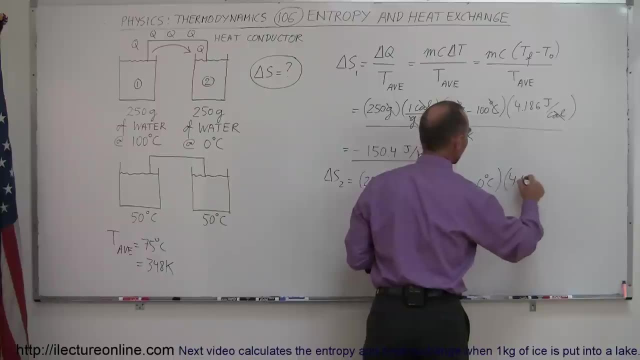 Kelvin. The difference now would be final temperature, which is 50 degrees centigrade, minus initial temperature, which is zero degrees centigrade, times a conversion factor four point one, eight, six joules per Kelvin, and then the whole thing divided by the average temperature. 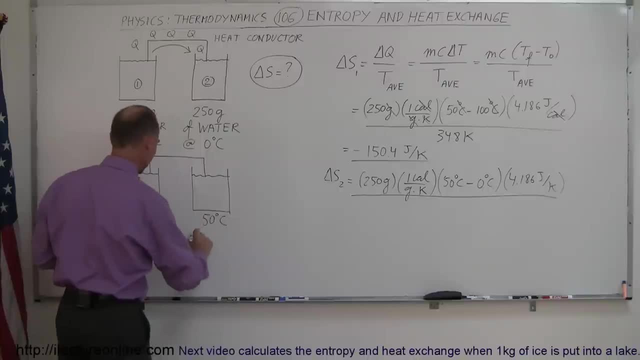 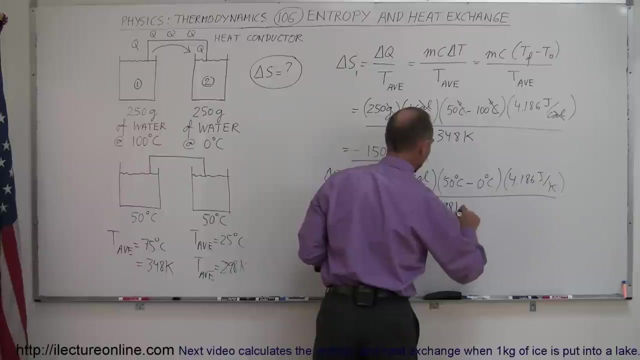 for the cold cup. Now that would be from zero to 50. So T average in this case is 25 degrees centigrade. That means the average in that case is two hundred and ninety eight Kelvin. All right, So that goes down here: Two hundred and ninety eight Kelvin. 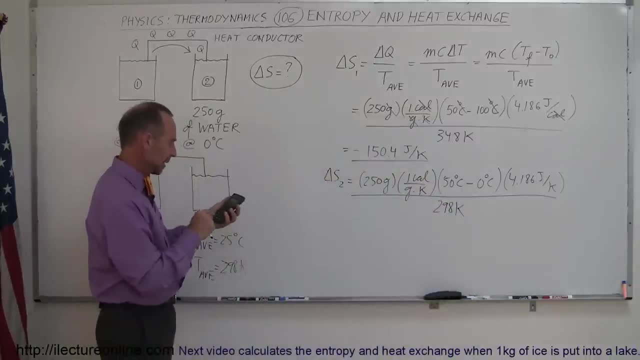 So let's figure out what that is equal to. We got 250 times 50. That's a positive 50 times four point one, eight, six, and divided by two hundred and ninety eight, And here we get Delta S two. And let me write here Delta S one. 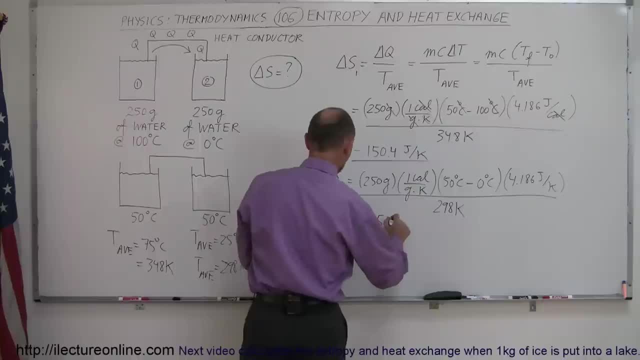 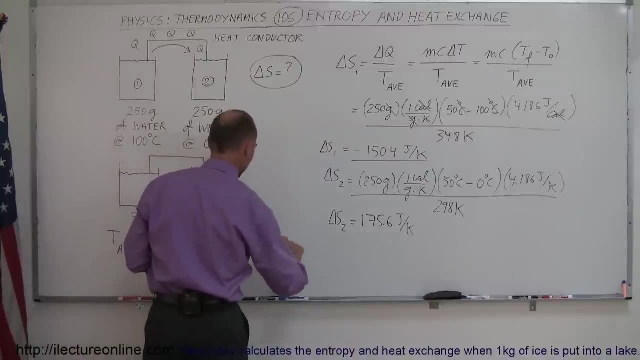 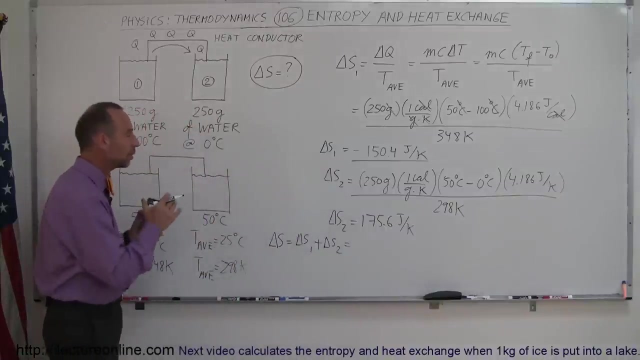 So we we compared is one hundred and seventy five point six joules per Kelvin. Now for the total change in the entropy Delta S. that is equal to Delta S one plus Delta S two. So what you could see here is that you have to add the entropy change of every piece. 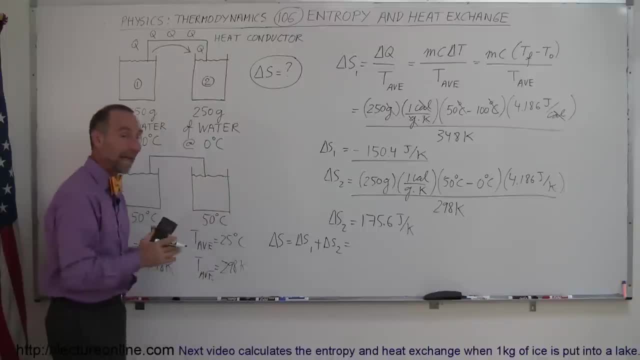 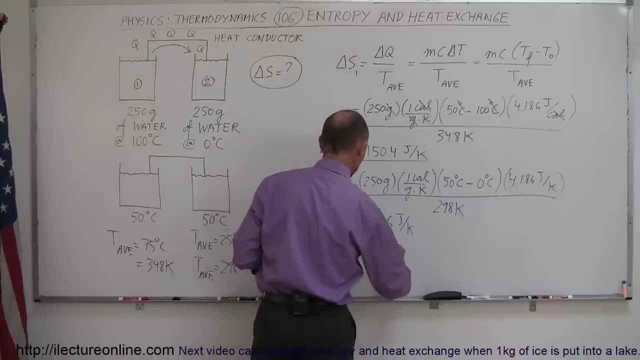 of that heat exchange in this case, or two cups of water. So we have to add the entropy change for both cups of water. So the first cup it was a negative change because he was removed. One hundred fifty point four joules per Kelvin plus the heat exchange here is positive. 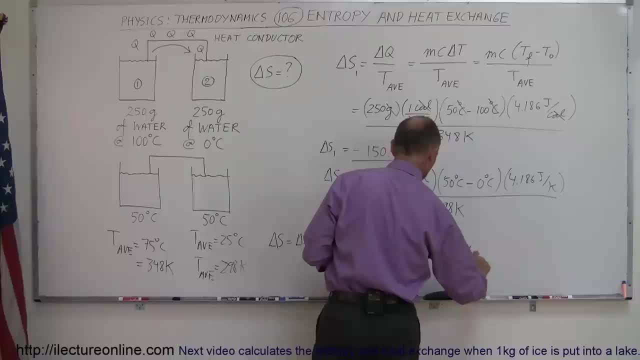 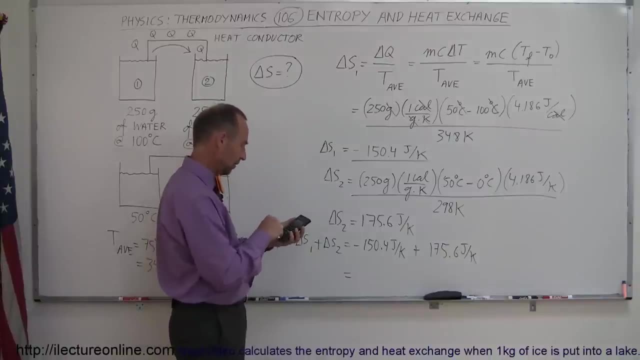 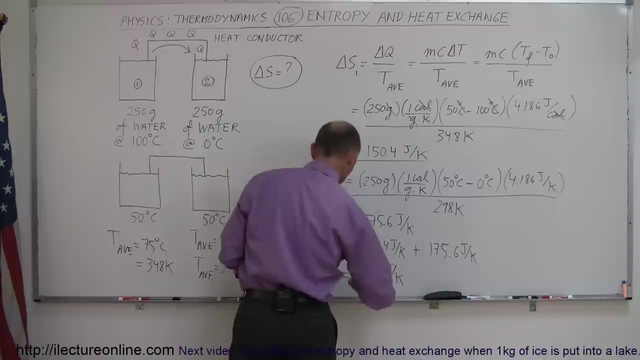 So we have 175.6 joules per Kelvin and that means we have 150.4 negative plus 175.6 positive, so we have a 25.2 joules per Kelvin, which is the delta S for this heat exchange. 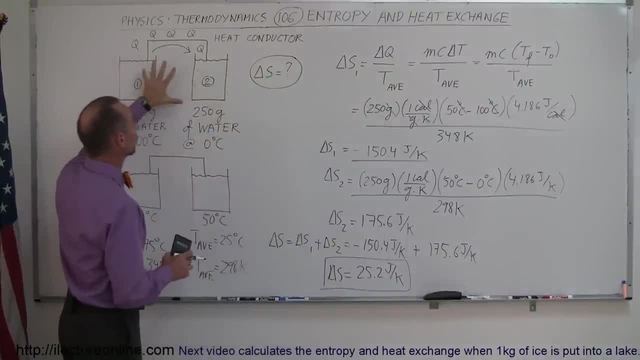 For the amount of heat that was exchanged from the hot cup to the cold cup, the universe's entropy increased by 25.2 joules per Kelvin, which means that's how much less available energy is to do work after we exchange that heat. and that's how you do that problem. 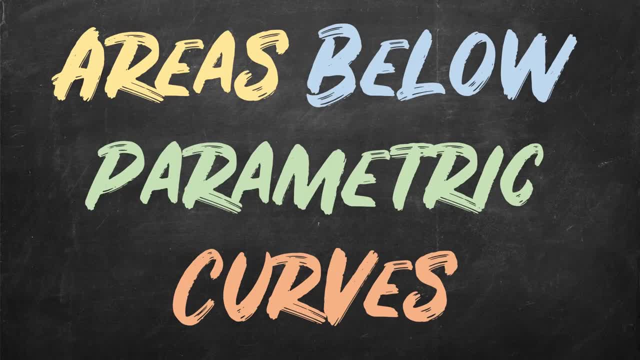 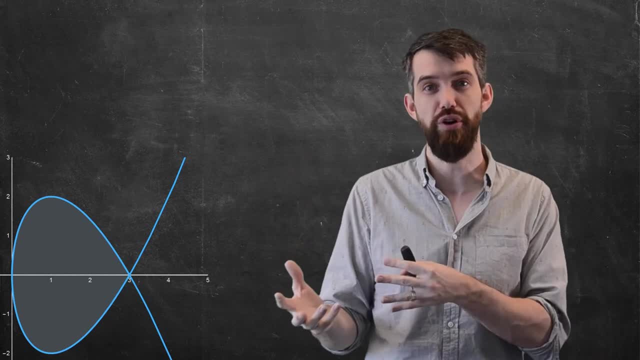 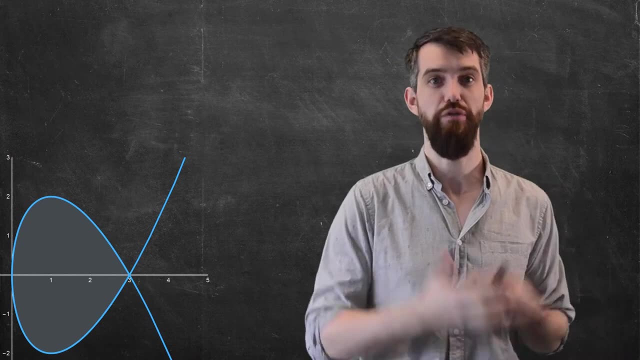 In our second video on how to take things we've done before in calculus and apply them in the context of a parametric curve, we're going to look at areas enclosed by some particular curve, That is, in this case. I have this parametric curve that we saw in the previous. 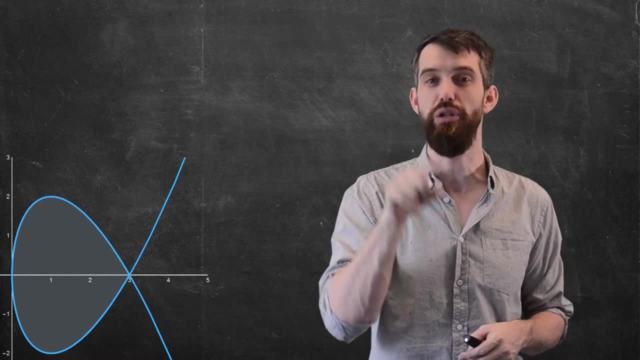 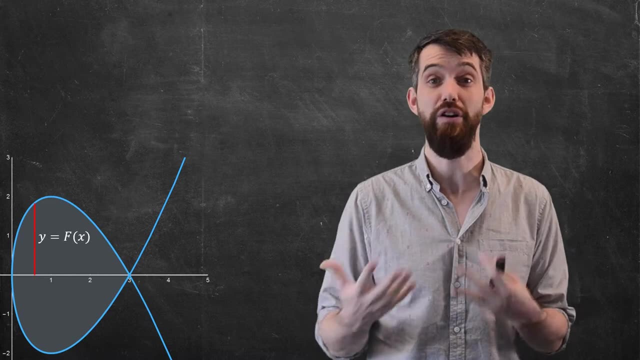 video. and now I'm interested in what is the area inside of that little loop? Well, recall that we've done areas before and what we usually did back in the day was write it as y is a function of x and that we describe this height as going from the x axis up to 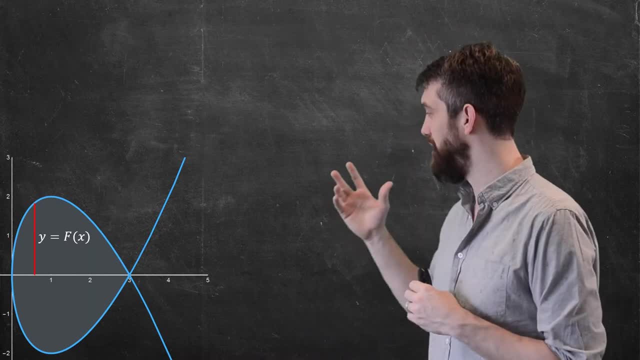 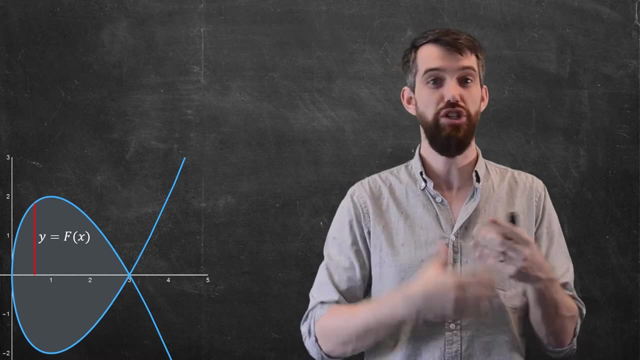 whatever our function was. So if I just, for example, take the positive half of this, maybe multiply by 2, by symmetry at the end, but just take the positive halves, then that's just a familiar y is f of x, And then what we would typically say would be that the area 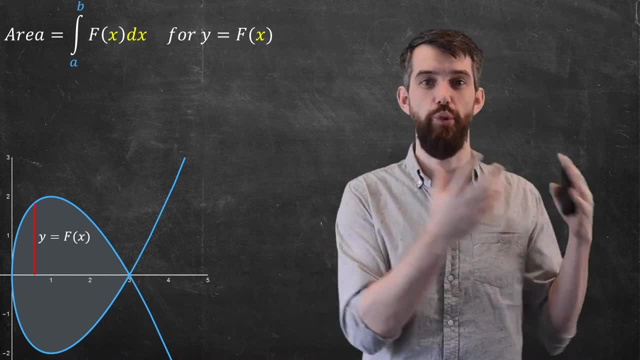 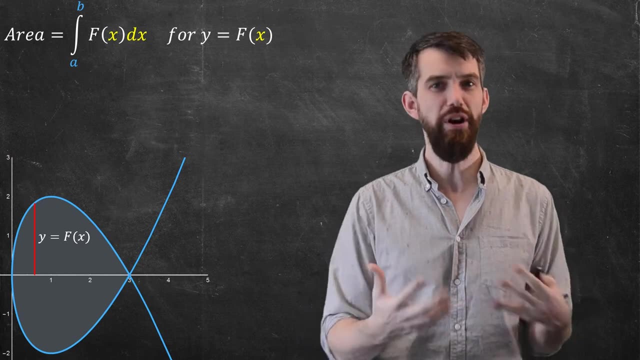 was going to be the integral from a to b, some left endpoint and some right endpoint, on your x values of the y, or in other words the f of x, dx. But what we're now going to be talking about is parametric curves where x is a function of t.